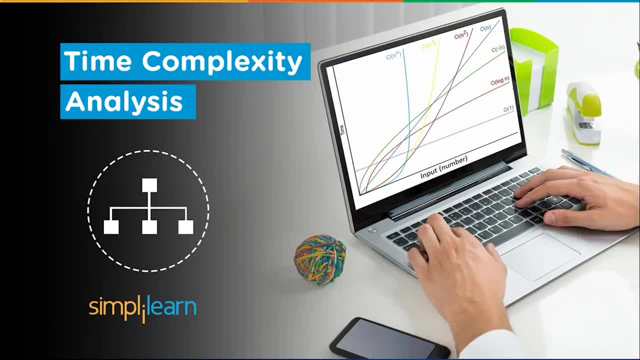 knowing how to evaluate them using time complexity can make the program behave in required optimal conditions. Doing so makes us an efficient programmer. On that note, hey everyone, I am Vibho Khandelwal and I welcome you all to yet another exciting video from Simply Learn. In this session, we will be discussing time complexity analysis. 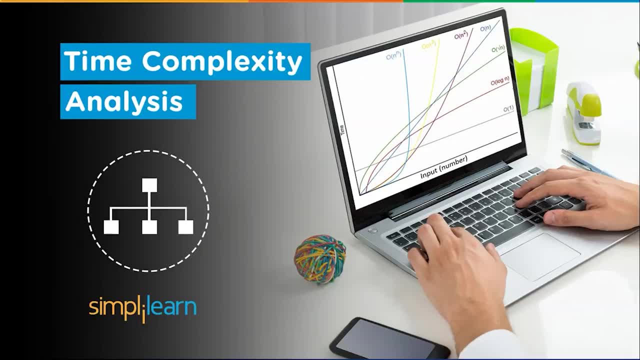 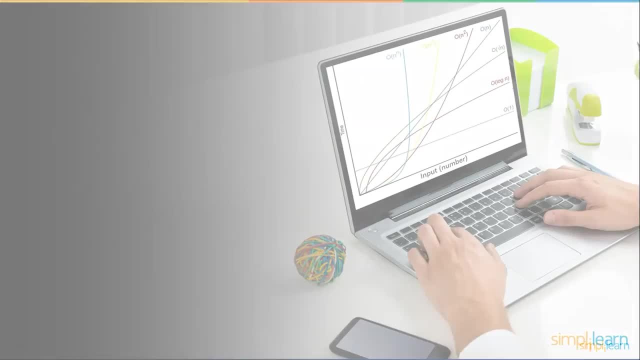 However, before we begin the session, make sure you have subscribed to our YouTube channel and clicked on the bell icon below so you never miss an update from Simply Learn. So now let's look at the agenda for today's topic. We shall begin our session by introducing. 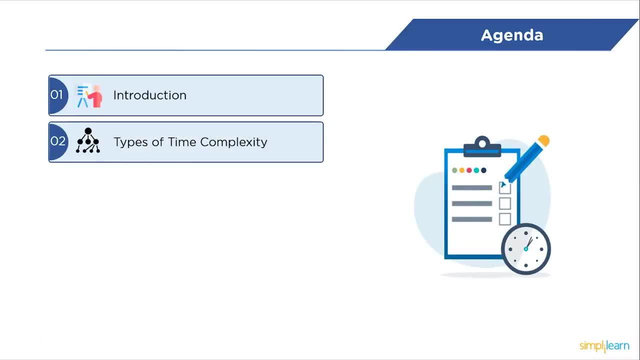 time complexity. Then we will discuss the types of time complexity And then we will discuss all the steps to evaluate the time complexity. Then we will briefly look at the time complexity of various algorithms. Finally, we will sum up what we have learnt. 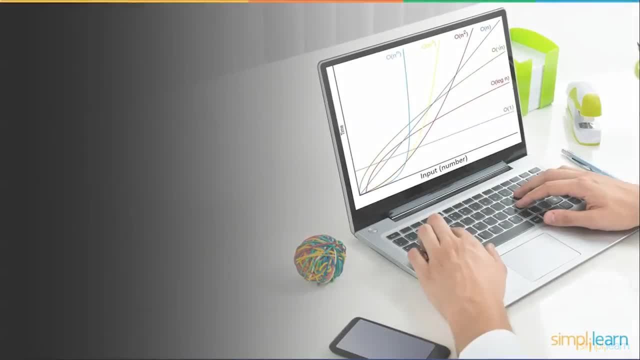 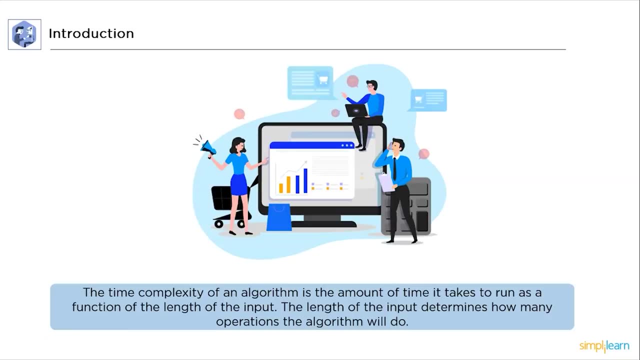 from this session. So, without any further ado, let's get started with the first topic of this session: introduction to time complexity. The time complexity of an algorithm is the amount of time it takes to run as a function of the length of that input. The length of the input determines how many operations the 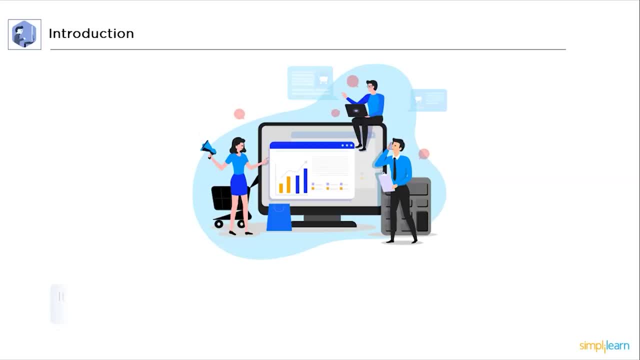 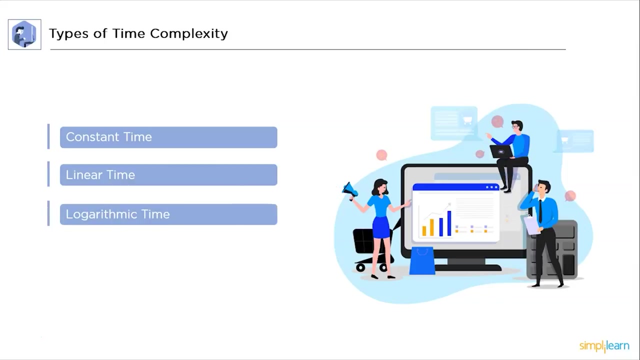 algorithm will do. It will provide the information about the variance, increase or decrease in execution time as the number of operations in an algorithm increases or decreases. Next we will discuss the types of time complexity. We will start with the constant time complexity, Then we will discuss linear, logarithmic, quadratic time complexity. 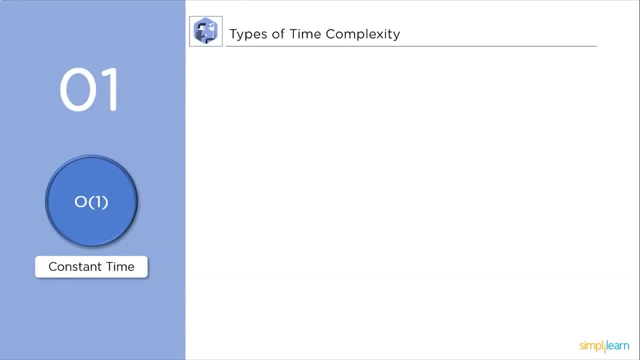 Now let's have a look at them in the detail. First, constant time complexity. When an algorithm is not reliant on the input size n, it is said to have a constant time of order bigger or smaller than 1.. The runtime will always be the same, regardless of the input. As you 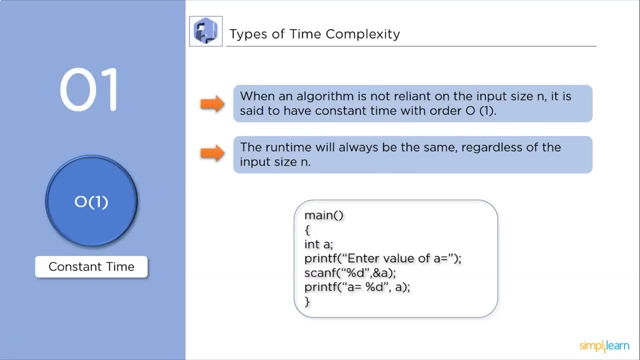 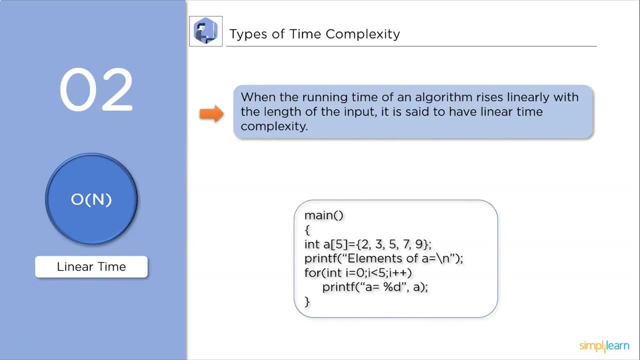 can see in the code, every line has the runtime of 1.. And they are all independent of any input size, so the runtime is always constant. Next up, linear time complexity. When an algorithm's running time increases linearly with the length of the input, it is said to have linear time. 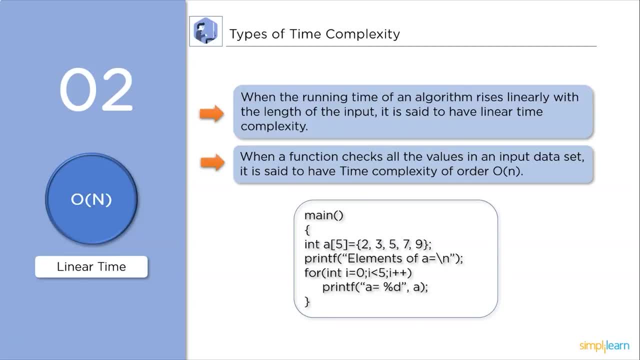 complexity. When a function checks all the values in an input dataset, it is said to have the time complexity of order of bigger or smaller than 1.. As you can see in the code, the loop depends on the size n. So the time complexity rose up to n. 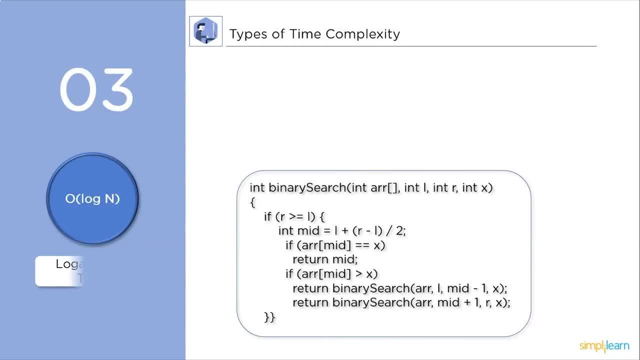 Next up, logarithmic time complexity. When an algorithm lowers the input data in each step, then it is said to have the logarithmic time complexity- Goodbye. As you can see in this code, by finding out the mid in every iteration, the runtime will. 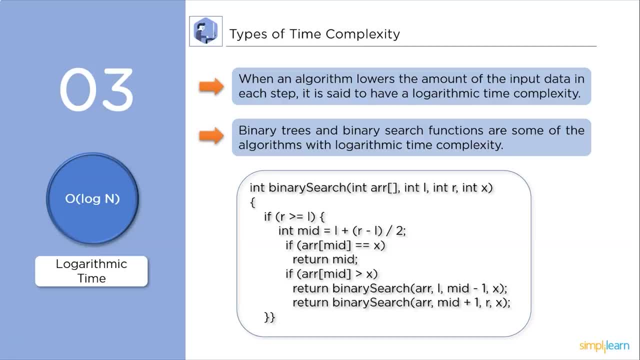 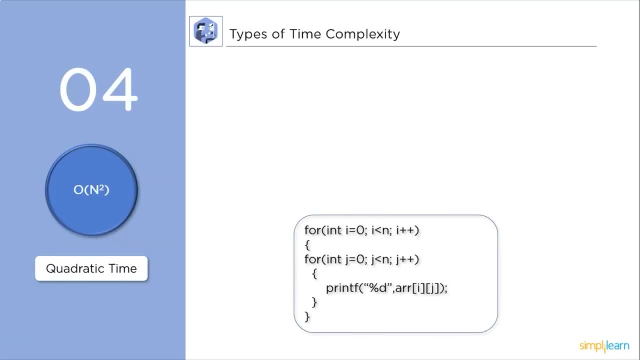 decrease every step, making it approximately logarithmic runtime. Next up: quadratic time complexity. When the execution time of algorithm rises non-linearly up to n square with the length of the input, it is said to have the quadratic time complexity. Next up quadratic time complexity. When an algorithm's running time increases non-linearly. 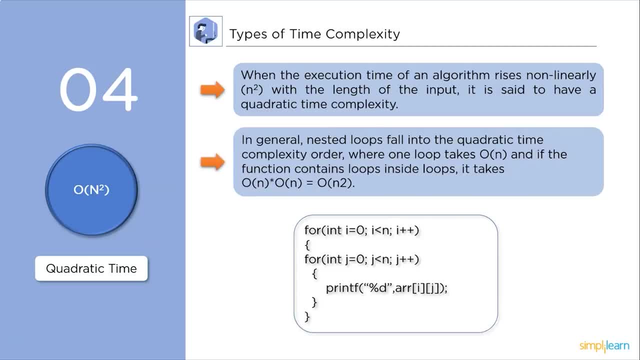 between n and 2, it is said to have the logarithmic time complexity. Then the runtime will look. complexity in general net nested loops falls into the quadratic time complexity order, where one loop takes bigger of n and if the function contains the loop inside the loop then it multiplies. 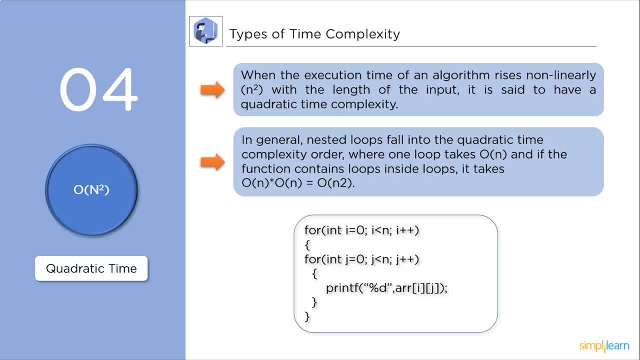 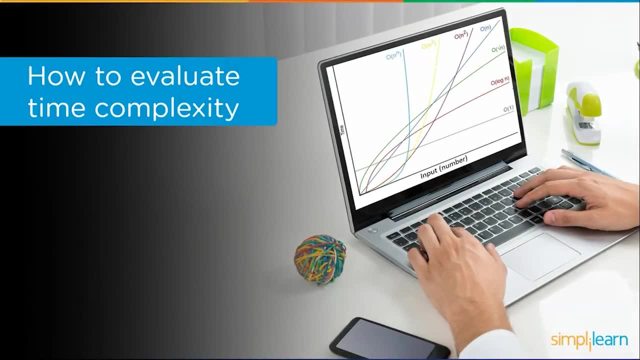 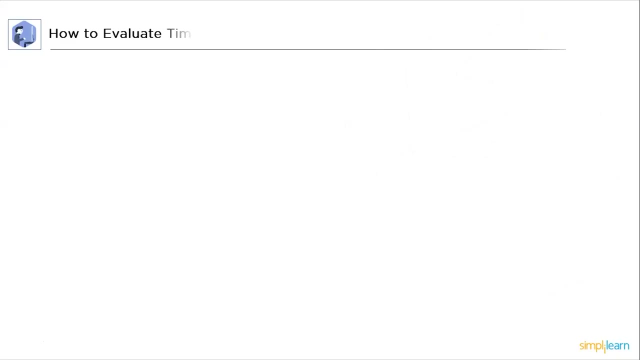 as you can see in this code, because of the nested loops, the time complexity rose to n square. now that you have the firm grasp of time complexity and its type, we will discuss essential steps to evaluate the time complexity. to understand this, we will take an example of fibonacci number. this code prints the: 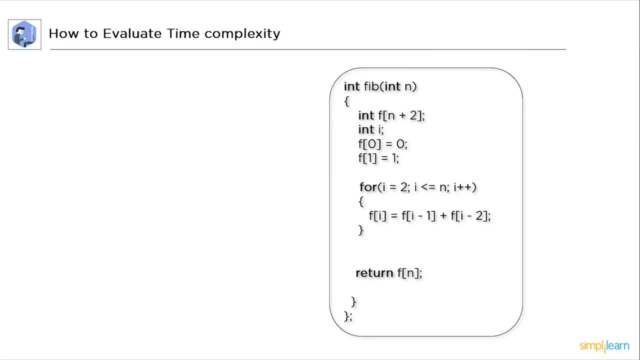 fibonacci numbers till n. we will divide this code into three parts, isolating all the loops that play a significant role in altering the time complexity. let's look at the first part. it consists of some independent statement which gave constant runtime for each statement. next let's move. 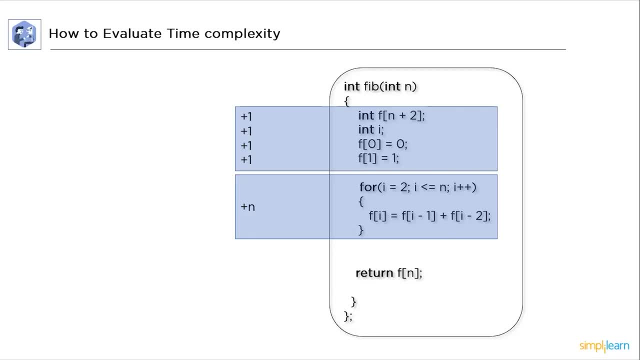 onto our next part, that is, for loop. Since this loop runs n times, this will give linear time complexity on n. Next up the third part, which also has the constant time complexity. Now let's take a total of runtime which comes out to be n plus 5.. We will then discard the. 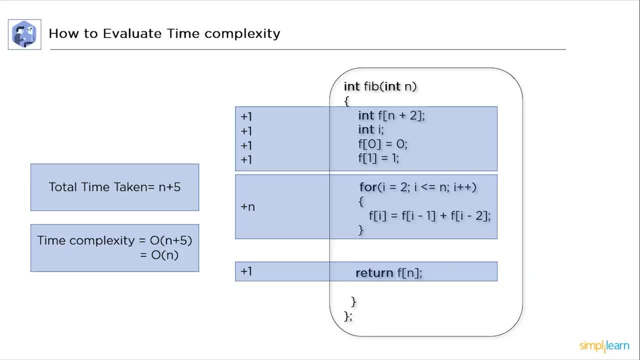 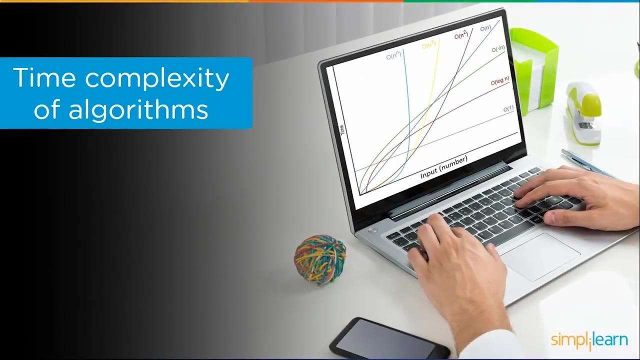 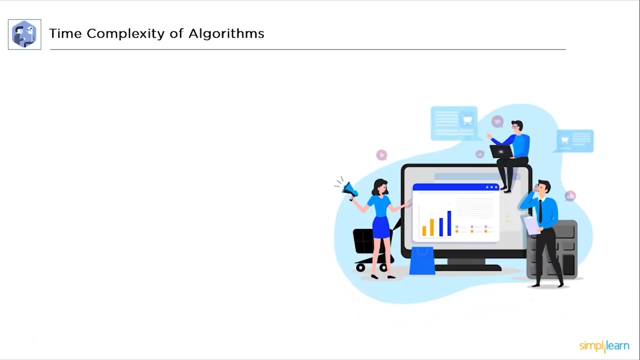 constant part to find the time complexity which does not affect the overall time complexity. Now we will have the final time complexity of O. We have now discussed time complexity and how to evaluate it. Now let's have a look at the time complexity of various algorithm. We will look at the time complexity of insertion. 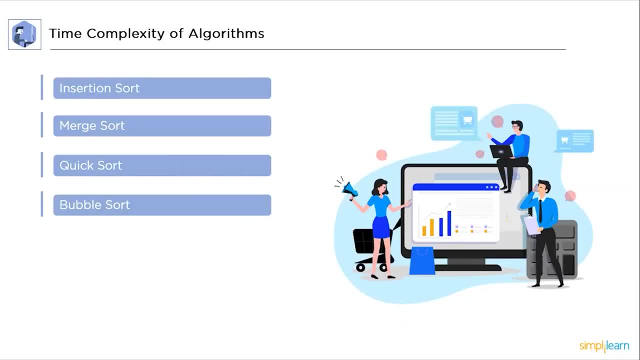 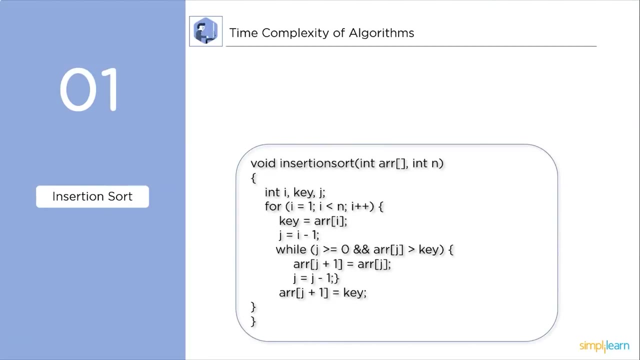 sort, merge sort, quick sort, bubble sort and some searching algorithms like linear search and binary search. Let's look at the them in the detail. First up, insertion sort. As you can see in this code we are using nested loops, So in worst case its complexity comes out to be n square. Now, in the best, 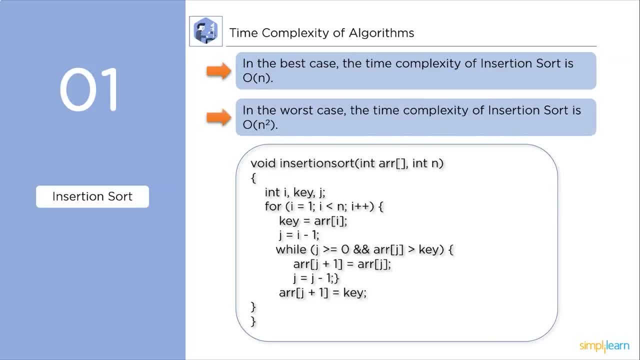 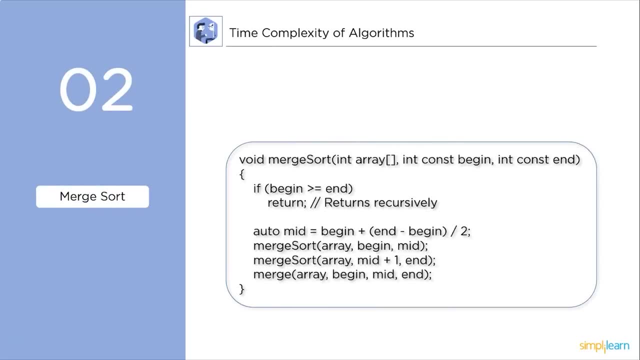 case scenario, the complexity will be linear time complexity. Next up merge sort. In this case, whether it is the worst case or the best case, it will always remain n log n, as every statement in this code will run the same amount, So no matter what its time. 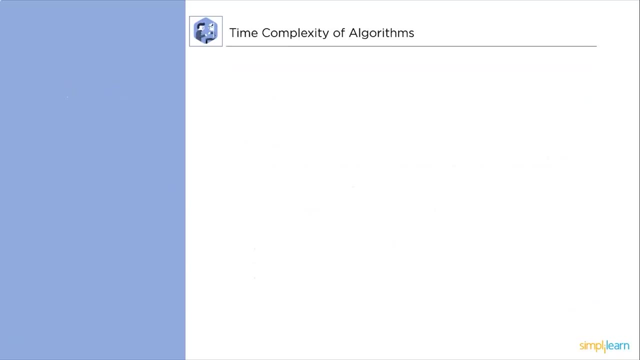 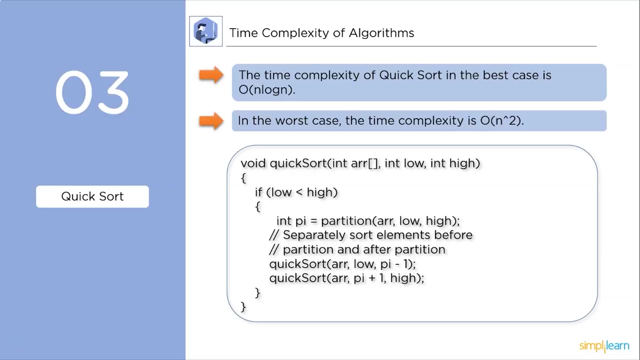 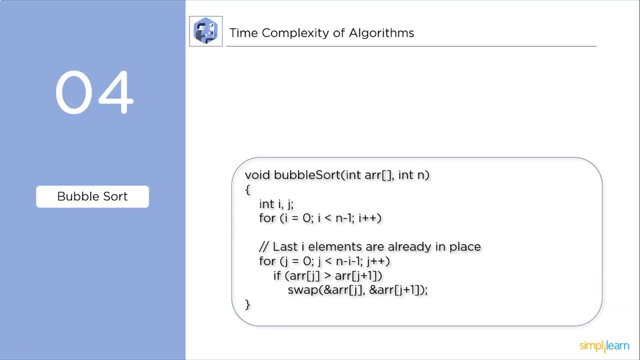 complexity will remain the same. Next up quick sort. The time complexity of quick sort in the best case is n- log n and in the worst case it is n- square. Next up bubble sort. As you can see, in this code we are using nested loops, So in the worst case scenario, 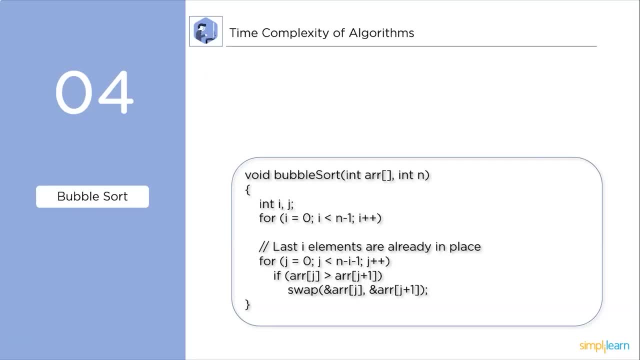 its complexity comes out to be n square. Now, in the best case scenario, the time complexity will become the linear time complexity, that is, n, And after that we will discuss some of the searching algorithms. First up, linear search. In the best case scenario, if the 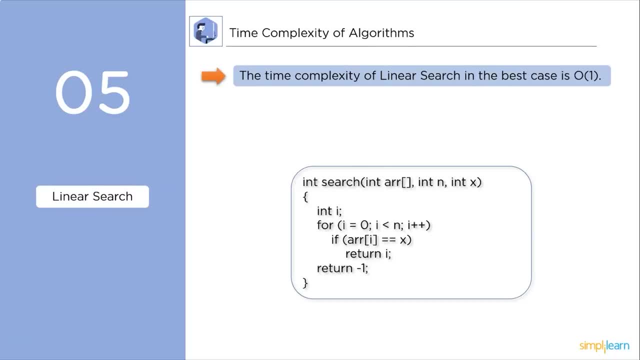 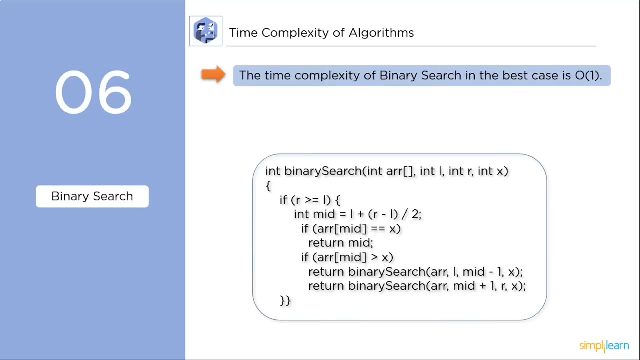 statement to be searched is at the first position, then the time complexity will come out to be constant, Whereas in the worst case, the time complexity will come out to be n. Finally, binary search. In the best case scenario, if the element 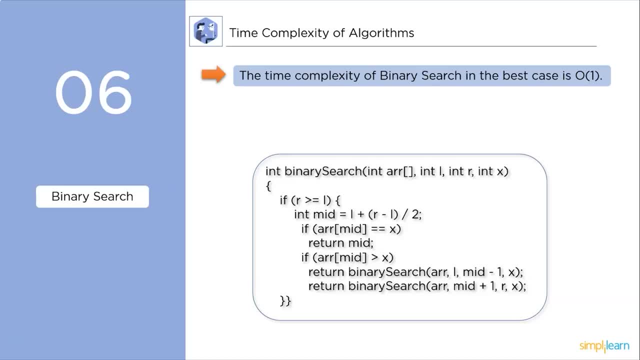 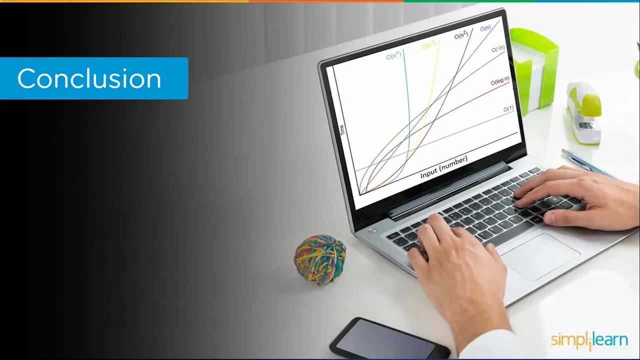 is to be searched is at the mid, then the time complexity will come out to be the constant, Whereas in the worst case scenario, the time complexity will come out to be Vega of log n. We have now discussed the time complexity and how to evaluate and the time complexity.